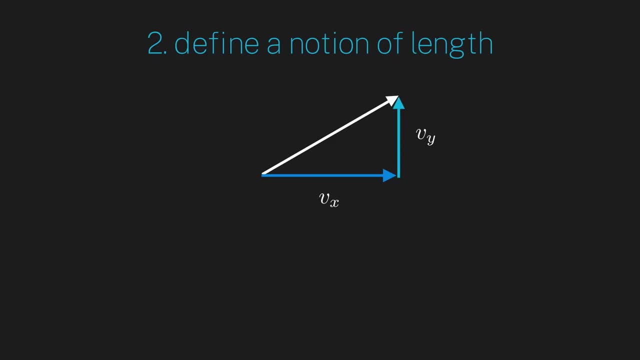 With our typical arrow approach. we can calculate the length of a vector using the Pythagorean theorem. Note that this is the same as the square root of the dot product with itself, so we can define it in terms of the dot product. Defining the length of a vector in terms of the dot product is really useful, since 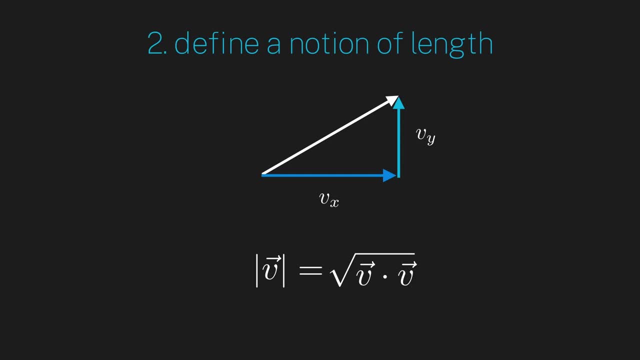 it can be used on vectors that aren't necessarily arrows. These are notions that we would like within our quantum vector space, So we want to find a way to take the dot product and abstract it to a concept that we can use in any vector. 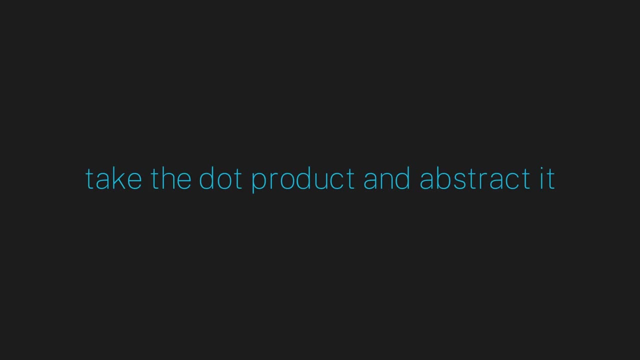 space, not just arrows and columns of numbers. This is exactly what the inner product is. So how should we define the inner product At its core? the inner product is a map that takes in two vectors and spits out a number. 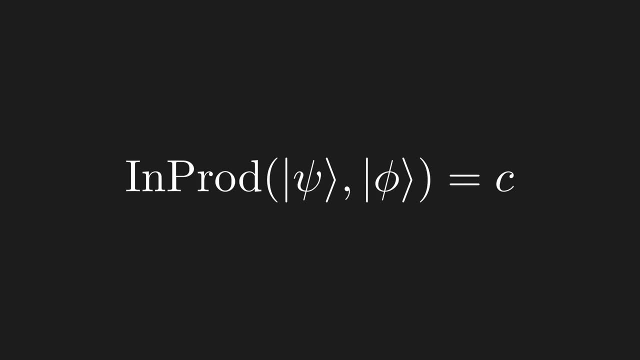 which might be complex. Now this notation is sort of clunky and in quantum mechanics we put a much cleaner notation for the inner product, which is done by putting two kets together, as shown- Really quick. I have one more thing to add before we define the inner product With looking. 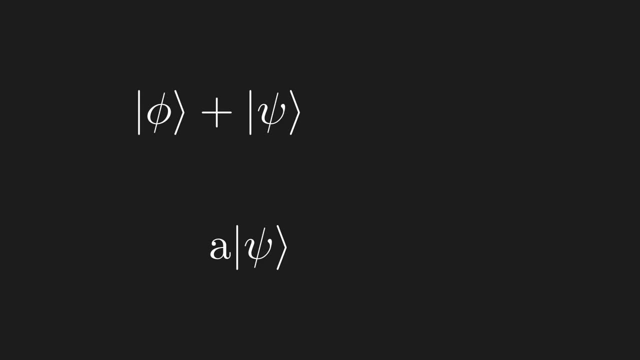 at addition and scalar multiplication of kets. it is common, and sometimes useful, to write them as a new ket, like this: This might seem weird at first, but once you've defined the inner product you can start to see the difference in the notation. So let's take a look at the inner product. At its core, the inner product is a map that takes in two vectors and spits out a number which might be complex. So let's take a look at the inner product. At its core, the inner product is a map that takes in two vectors and spits out a number which might be common. 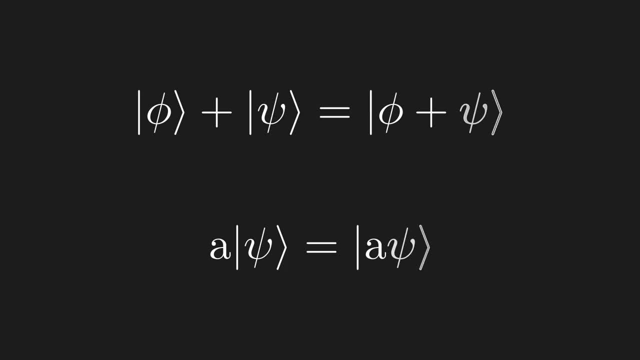 and sometimes useful to write them as shown. So let's take a look at the inner product, But consider it a label for the new vector that resulted from the operation shown Now. remember that we want an inner product in order to define things like length, which 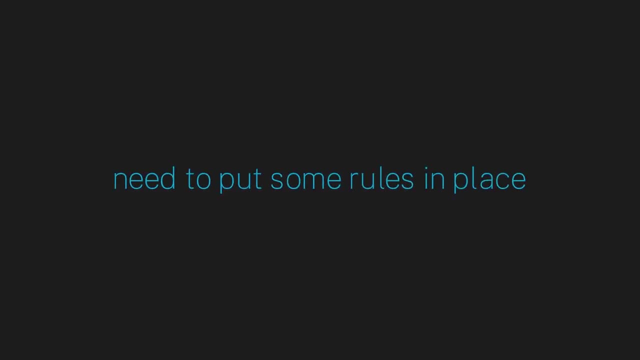 should be a real positive number. In order to do this, we need to put some rules in place. First, the inner product should be linear in the right hand position, meaning for kets, psi, phi and zeta in scalar a we have the following: 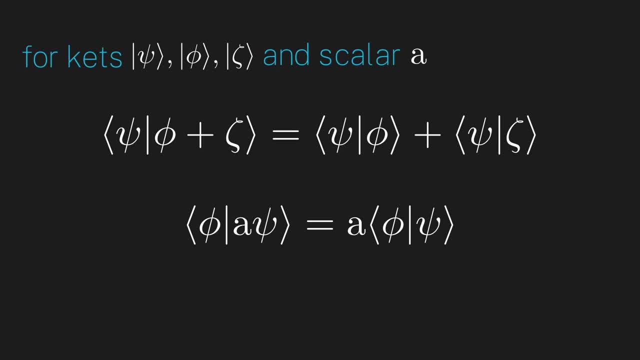 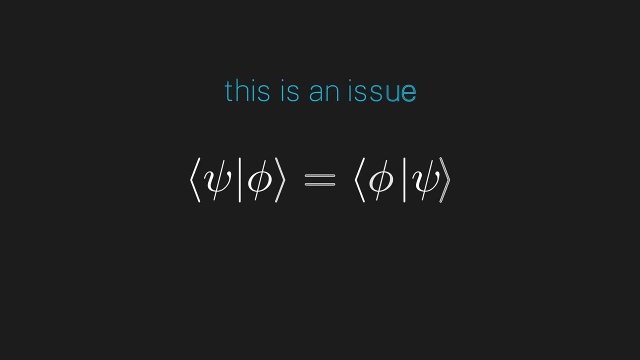 This just follows our intuition from the dot product. In a bit we'll show that we have a different rule for the left hand position. Next, what happens when we flip our inner product? meaning we do this. You might think we can just have it be equal, but let's see why this is an issue. 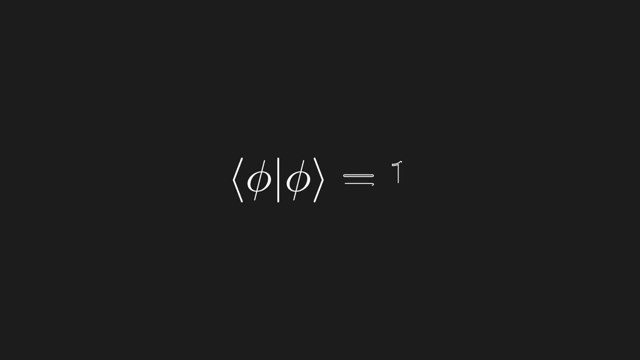 Assume the vector phi has an inner product with itself equal to 1.. Now let's calculate the inner product with itself of the new vector i times phi. We can take out the i from the right hand slot. Now, assuming flipping the inner product doesn't change anything, we can flip the two positions. 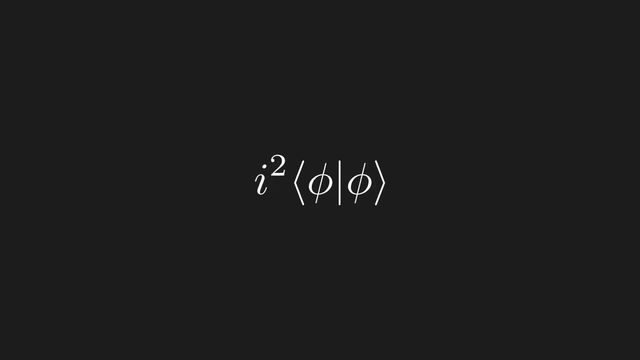 take out the i again and remember that we assumed the inner product equaled 1.. Thus we get that the new inner product is equal to negative 1, but this is a problem. Remember that we wish to define the length of a vector as the square root of the inner. 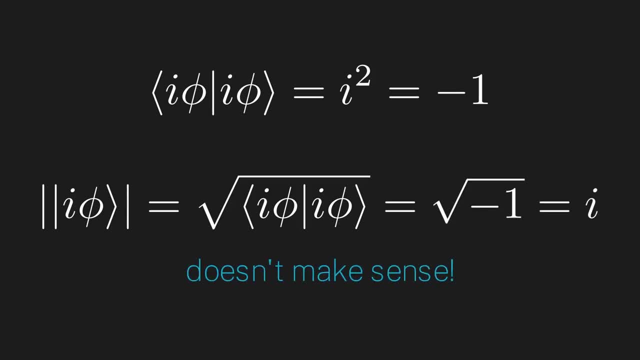 product with itself. In this case, we get an imaginary length, which doesn't make sense. The way we fix this issue is by adding the condition that when we flip the inner product, we must add a complex conjugate. If we go back into our previous example and add this condition, we now get the following: 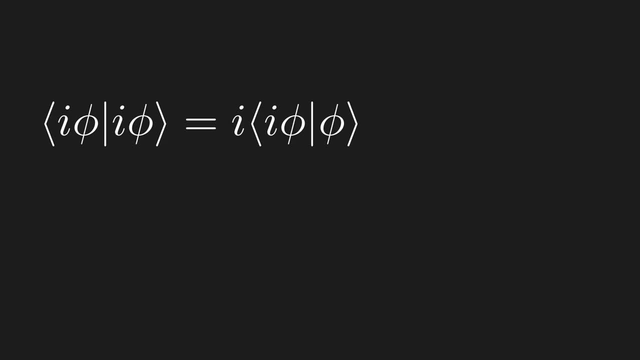 Take a second to follow each step. See how the complex conjugate gave us a 1 in the end, and hence a real vector length. Last, we need one more condition to ensure that the magnitude of vectors makes sense. We must impose the fact that only the zero vector has zero length. 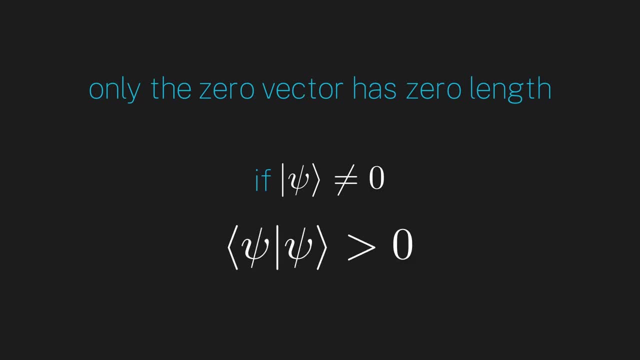 Meaning if your vector is non-zero, then its length must be greater than zero. Common sense right. And that's it. We now have the formal definition of the inner product. See how the complex conjugate gave us a 1 in the end and hence a real vector length. 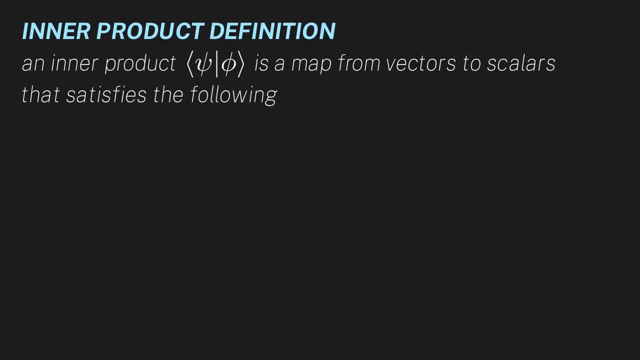 Do you now see how these conditions are just the dot product, with a few extra rules to make sure we can still define length? Hopefully the inner product is not so mysterious anymore. Now what if we had a linear combination on the other side of the inner product? 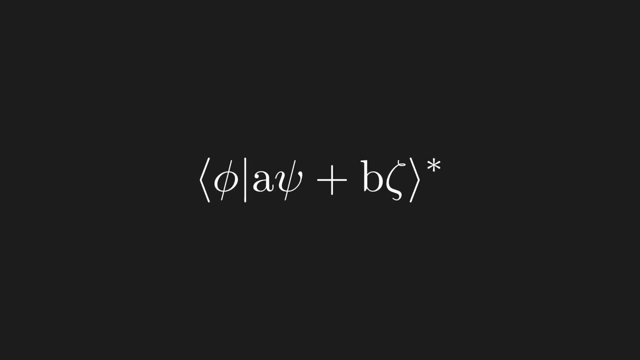 Well, we can just apply our current rules. We can first flip it, giving us the combination, Then we can use the linearity of the right slot, making sure to distribute the conjugate accordingly. Then we can flip the inner products again, which cancels out the conjugate. 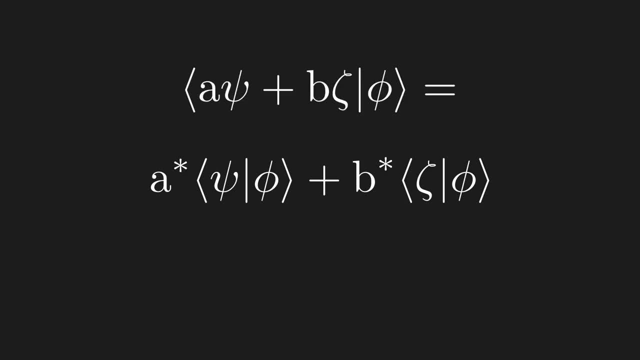 So what we get are inner products with conjugated coefficients. So, although the right slot acts linearly, the left slot acts what we call antilinearly, where the coefficients are conjugated. Great, Let's estimate. Okay, Let's establish a few more things about the inner product. 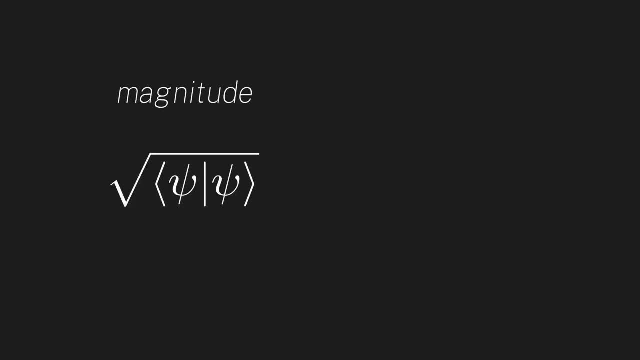 Following our intuition from the dot product, we will define the magnitude of a ket to be the square root of its inner product And we will say that two vectors are orthogonal if their inner product is 0.. With this, let's now use the inner product to see how it works in our quantum vector. 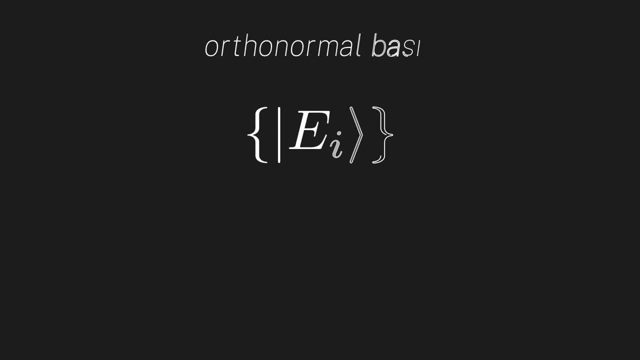 space. First, let's say we have an orthonormal basis, which means that each vector has length 1, and they are mutually orthogonal. Okay, So we can now estimate the magnitude of this vector to be 1.. It's common for physicists to combine these two conditions into 1 using the Kronecker. 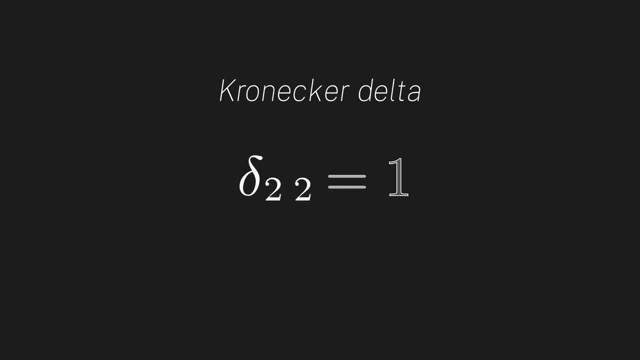 delta. The Kronecker delta is a very simple object with two indices. When the indices match, it equals 1.. And when they don't, it equals 0. So the orthonormal condition can be condensed into one statement. Check yourself to see that this is true. 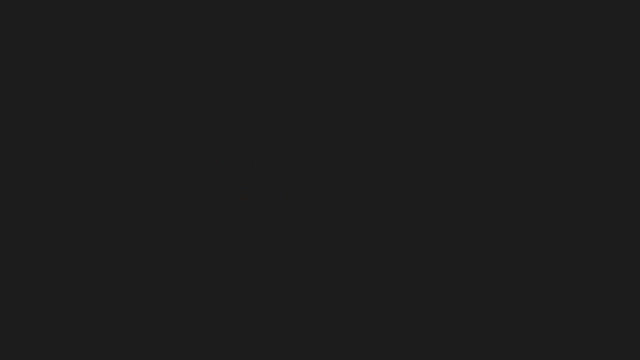 So if we have an orthonormal basis, we can expand in arbitrary order. We can also expand in arbitrary quantum state in this basis. Now, how would we get a particular coefficient? Well, because the vectors are mutually orthogonal, we can use the inner product to single out. 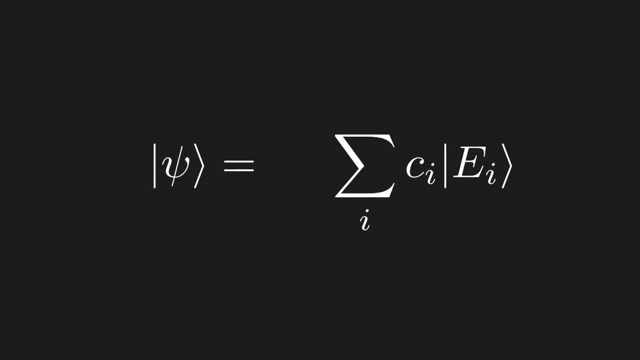 the coefficient that we care about. So if we want the second coefficient, let us take the inner product with the second basis vector. Using the fact that the inner product is linear in the right slot, we can move the inner product into the sum. 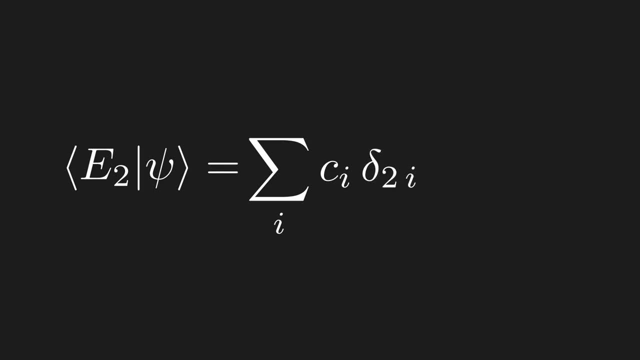 Now let's write the inner product as a Kronecker delta. Remember that the Kronecker delta is a constant, So we can use the inner product to single out the coefficient that we care about. The Kronecker delta only equals 1 when the indices match, equaling 0 otherwise. 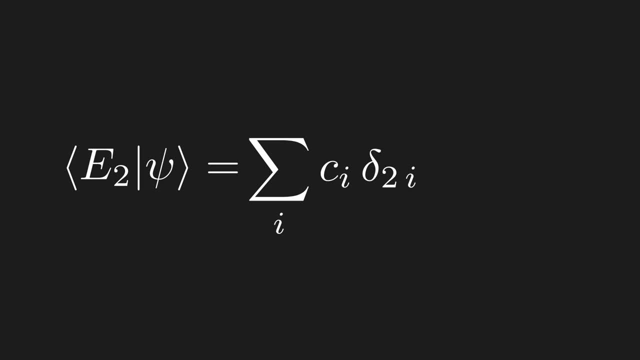 So when we sum over a Kronecker delta, all elements of the sum will be 0, except the one that matches the index. So what we can do is collapse the sum, and anywhere we see an i, we just replace that with a 2.. 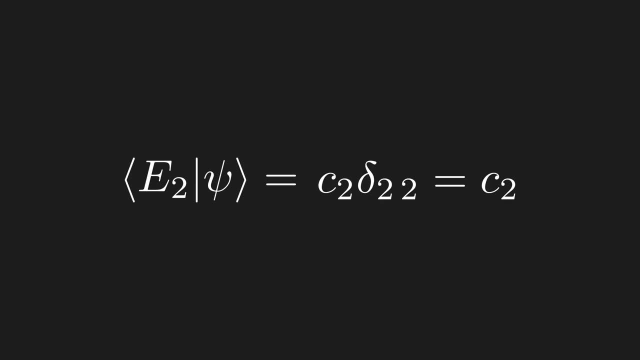 So what we get is our coefficient. It may have seemed excessive to use the Kronecker delta there, but trust me, it is a powerful tool to get used to. To see just how powerful it is, let's look at the inner product of two vectors. 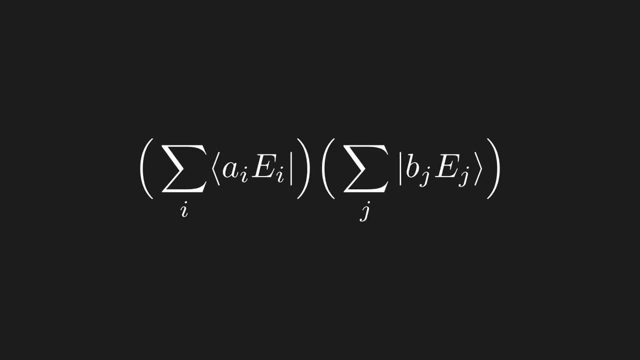 Like before, we expand both in an orthonormal basis. To simplify this, let's remember our rules. First, remember that the inner product of a sum of vectors is the sum of the individual inner products. So we get a double sum. 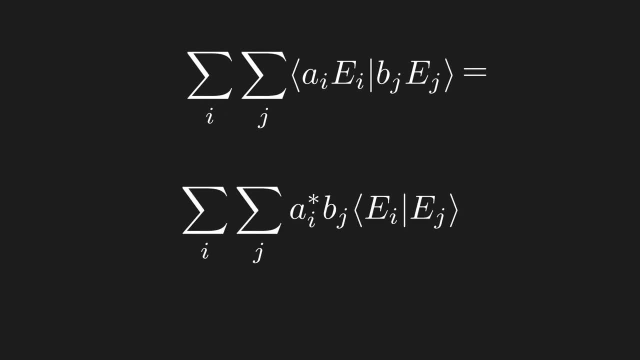 Next, remember that the right slot is linear, so we pull out the b coefficients And on the other hand, the left slot is antilinear, So we pull out the a coefficients and conjugate. We assumed this was an orthonormal basis, so we can write this inner product as a Kronecker. 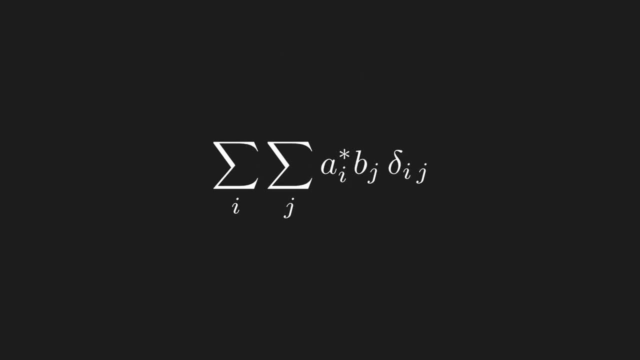 delta. Now remember what we said: The Kronecker delta is non-zero only when i equals j. So in the inner j-sum the only non-zero term will be the term that matches the i-index. So we can collapse the inner sum and replace j with i wherever we see it. 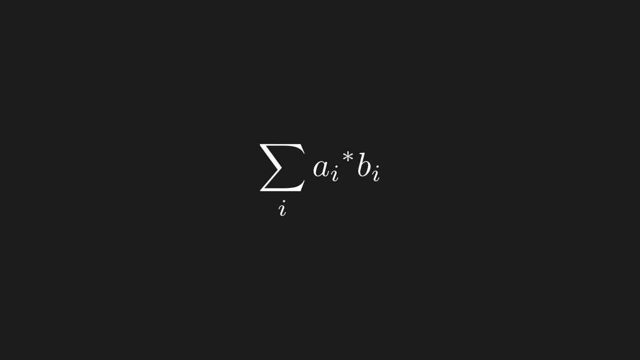 The remaining Kronecker delta just equals 1. So we get a double sum. See the technique. The Kronecker delta allows us to collapse sums easily. We just have to match the two indices. Awesome, and look at what we're left with. 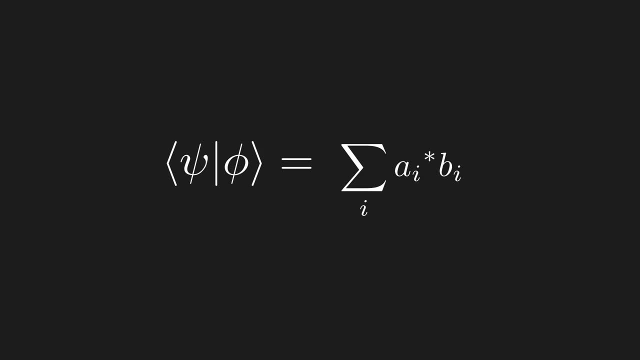 It may look weird, but let's say all the coefficients were real numbers. This means the conjugation doesn't do anything And we are left with the following: Look familiar, This is the dot product. We made no mention of the dot product in our definition of the inner product. 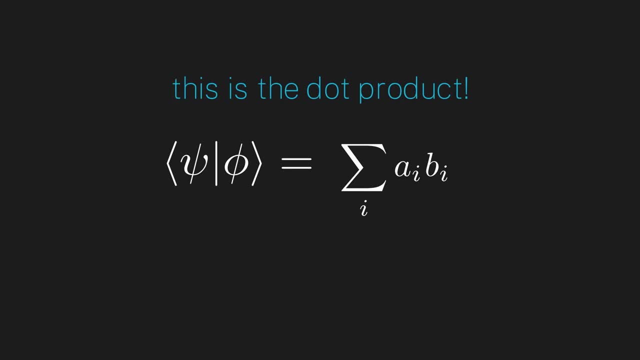 Yet here it is. So hopefully you see that the dot product is the dot product. So here it is. The dot product is what you get when you look at the inner product in a particular orthonormal basis. Now we have made a lot of progress with the inner product. 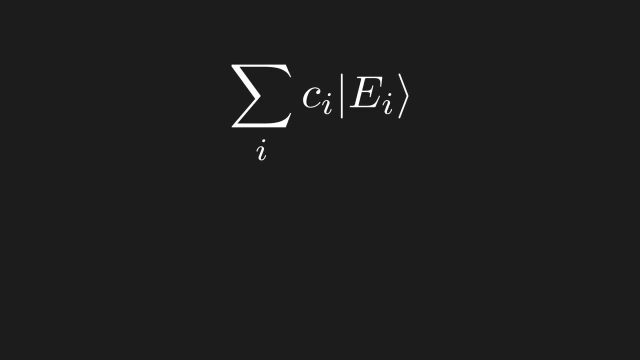 But so far we have only looked at the inner product with discrete linear combinations. What if we had a continuous linear combination, like we did when we looked at the linear combination of position outcomes in episode 2?? We will delve into this next episode where we will go in-depth on the Dirac delta function.